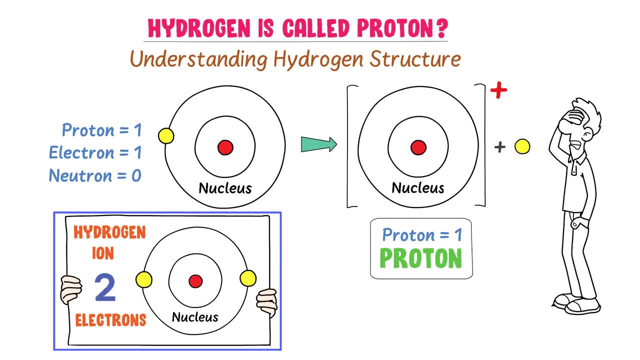 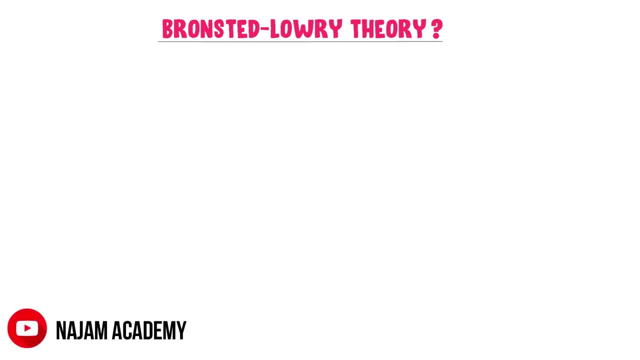 two electrons and its last shell, or valence shell. Now, what is Bronsted-Lowry theory of acids and bases? Well, according to Bronsted-Lowry theory, acids donate proton and bases accept proton. It means that acids donate hydrogen ion and bases accept hydrogen ion. For example, 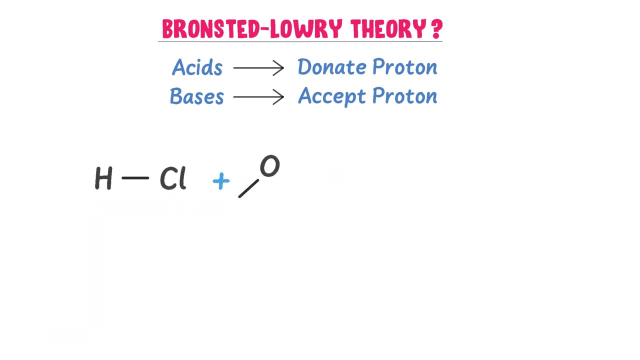 consider the aqueous solution of hydrogen chloride and water, We know that there is covalent bond between hydrogen and chlorine. So hydrogen and chlorine share one pair of electrons, But chlorine is more electronegative. So the shared pair of 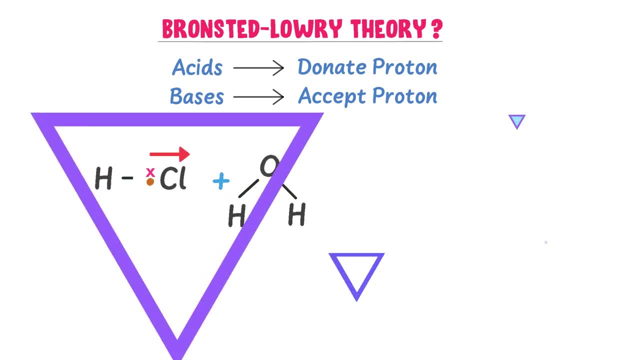 electrons is more towards chlorine than hydrogen. We also know that there are three long pairs of electrons on chlorine. Secondly, we know that there are two long pairs present on oxygen. Now listen carefully. This hydrogen will attack on the long pair of oxygen and would form a coordinate covalent bond with water. So the reaction is: 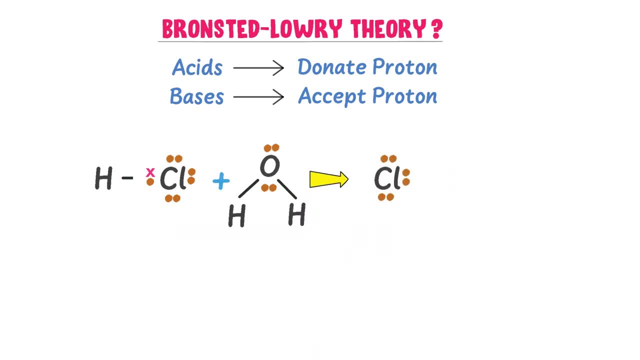 chlorine, three long pairs, and now it also carry the shared pair of electrons and this extra electron. So negative charge will appear on chlorine Plus oxygen, hydrogen, hydrogen and long pair on oxygen. We know that this long pair has been attacked by this hydrogen. 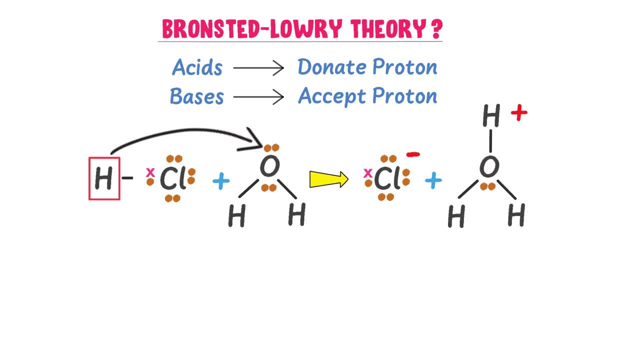 So we know that this hydrogen will attack on this oxygen. Now listen carefully. Hydrogen chloride has lost hydrogen, or more precisely, hydrogen chloride has donated proton. According to Bronsted-Lowry theory, hydrogen chloride is an acid, So we say that hydrogen chloride is. 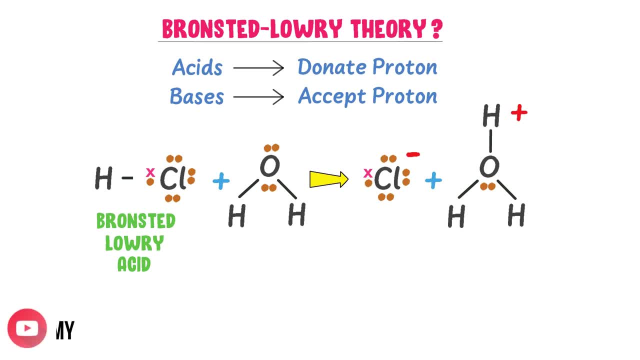 Bronsted-Lowry acid because it can donate proton. Secondly, we can see that water, chlorine and water has gained hydrogen ion, or more precisely, water has accepted proton. So we say that water is Bronsted-Lowry base because it can accept proton Also. a lot of students are very confused.